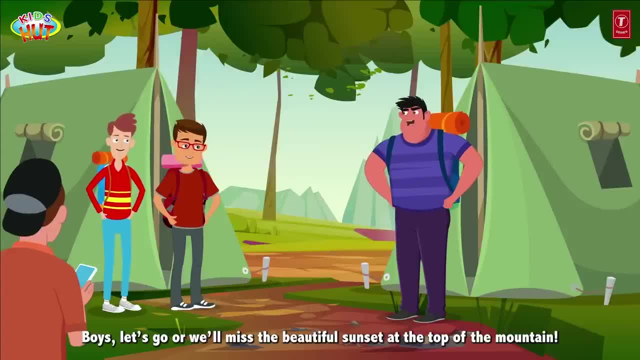 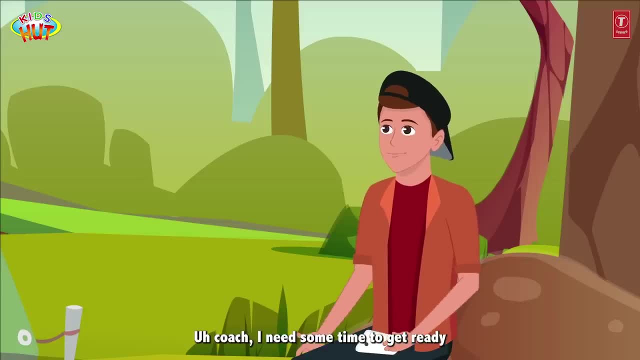 Always, always, Boys, let's go, Or we'll miss the beautiful sunset at the top of the mountain. Yes, sir, Let's go. Oh, coach, I need some time to get ready. You should have been ready by now, Oliver. 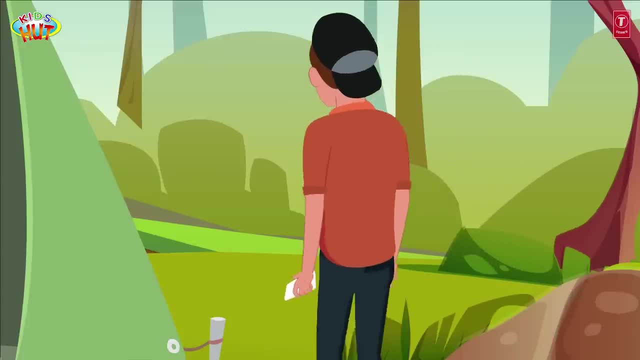 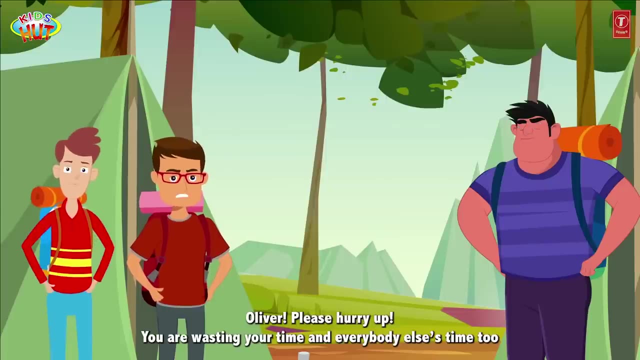 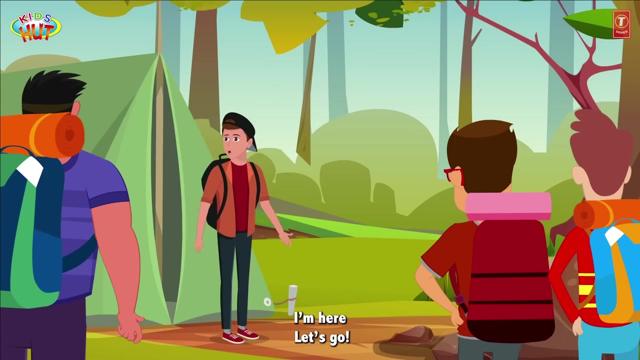 Come back fast. We are waiting for you. Yes, sir, Oh, Oliver, Please hurry up. You are wasting your time finishing the course. Everybody else is time too. We can't wait for you anymore. I'm here, Let's go. 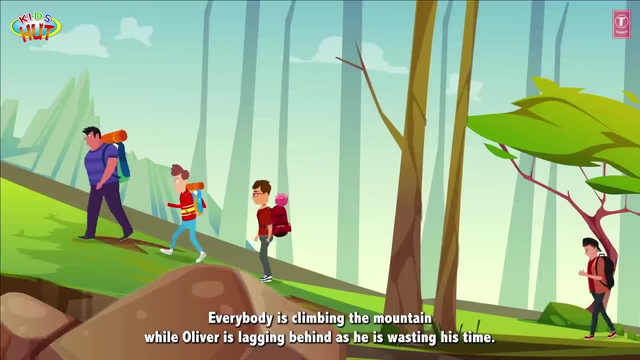 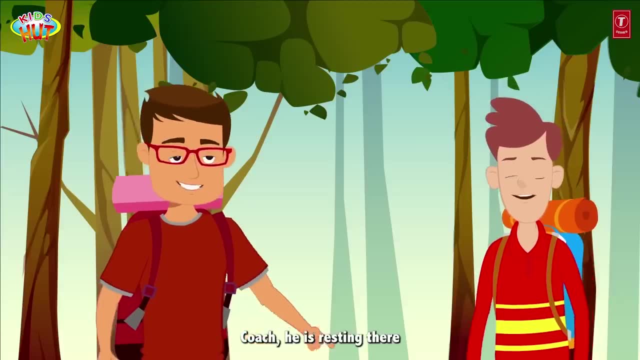 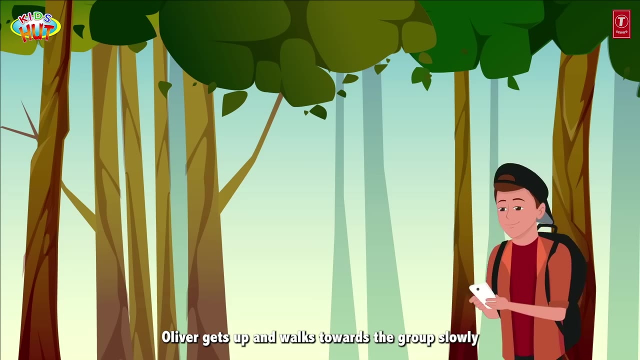 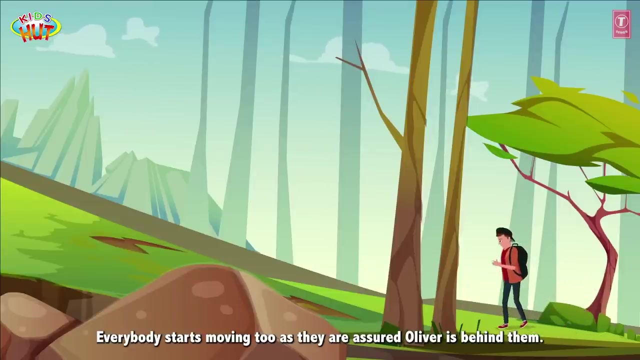 Everybody is climbing the mountain, while Oliver is lagging behind as he is wasting his time. Where is Oliver? I can't see him. Coach, he is resting there, Oliver, hurry up. Oliver gets up and walks towards the group. slowly. Everybody starts moving too, as they are assured Oliver is behind them. 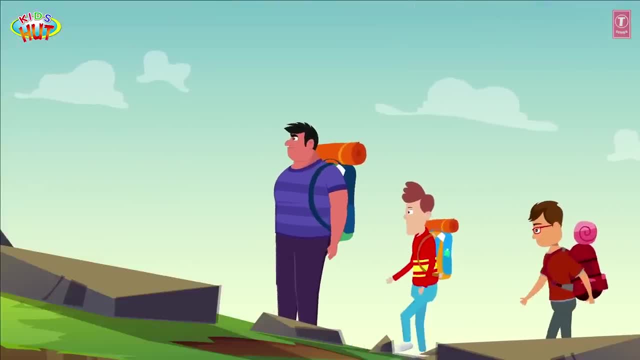 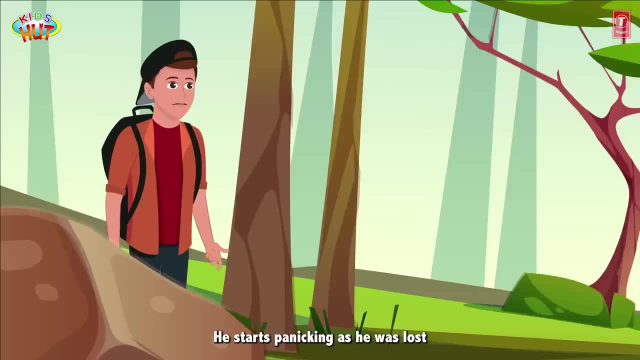 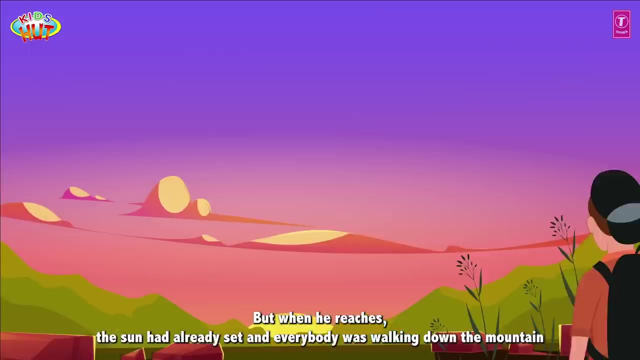 As everybody is climbing the mountain, Oliver loses track of the group again because he was wasting his time. He starts panicking as he was lost. He somehow finds his way and reaches the top of the mountain, But when he reaches, the sun had already set and everybody was walking down the mountain. 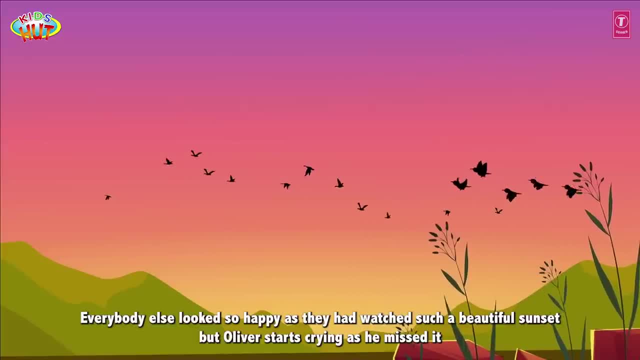 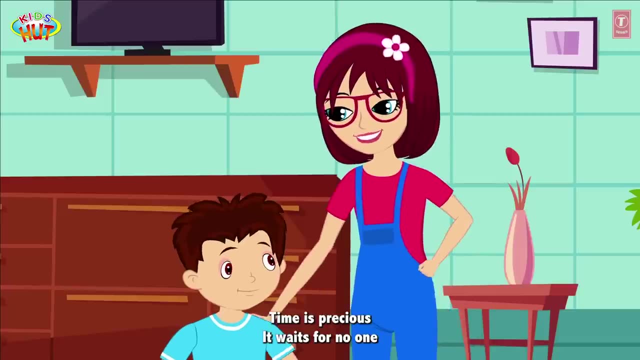 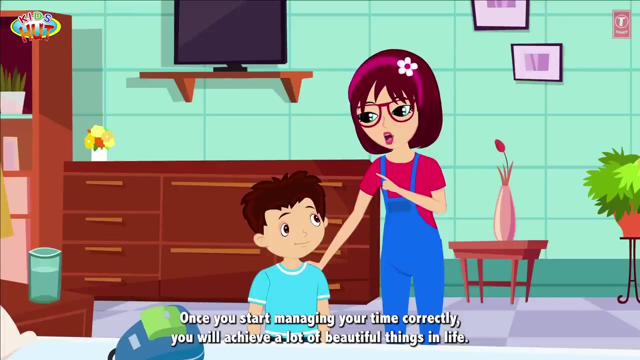 Everybody is moving too. Everybody else looked so happy as they had watched such a beautiful sunset, But Oliver starts crying as he missed it. Time is precious. It waits for no one. Once you start managing your time correctly, you will achieve a lot of beautiful things in life. 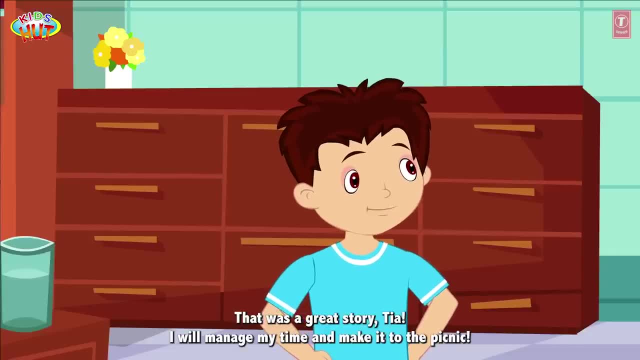 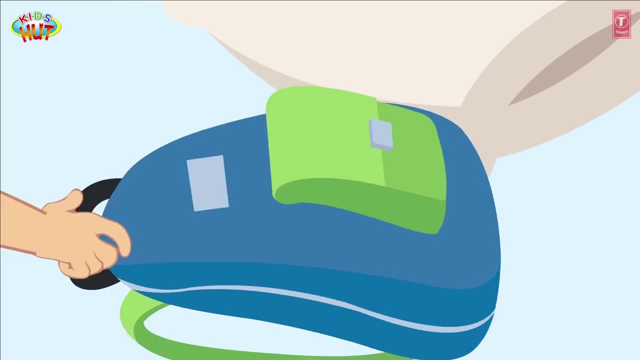 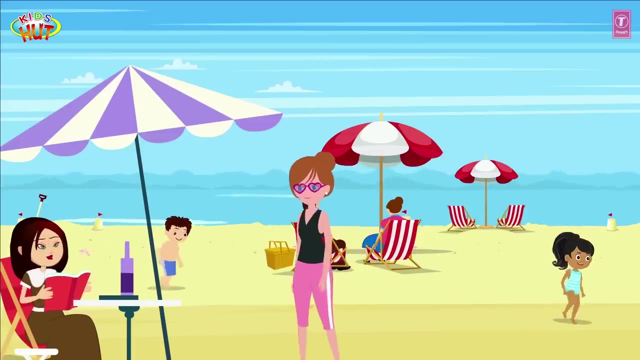 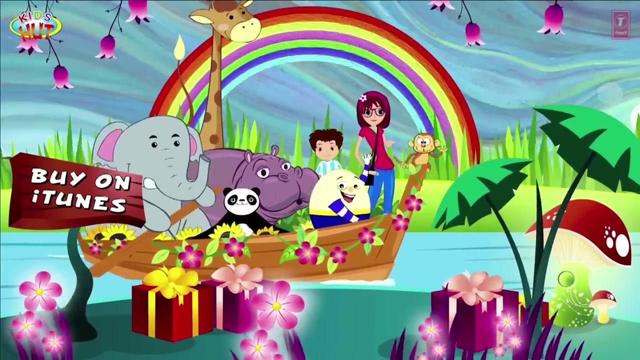 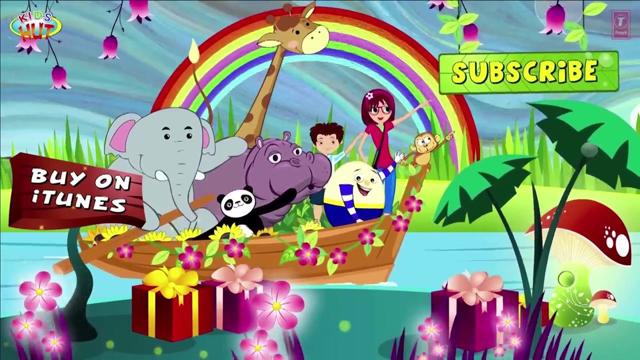 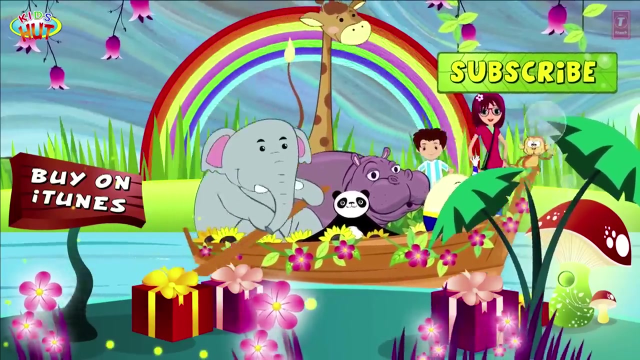 That was a great story, Tia. I will manage my time and make it to the picnic. Yes, Tofu, Now come fast or you will miss your school bus. Come on, let's go. Thank you,